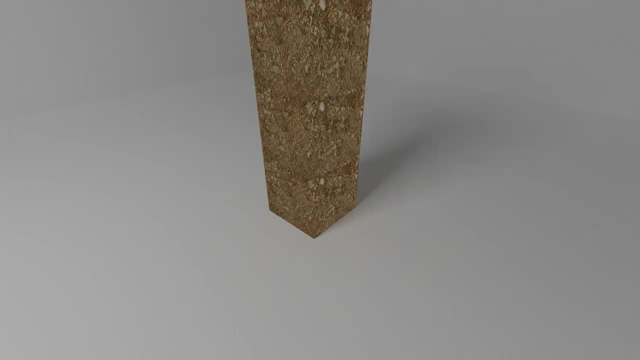 which is the vertical stress caused by the weight of the overlaying rocks and fluids on top of this cube up to the surface, And we call this overburden stress. There are also two other horizontal components of the stresses, which are caused by several parameters which we will explain later, of course. 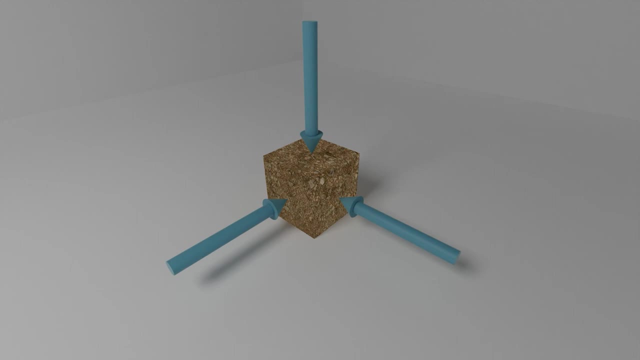 With one component bigger than the other. so we call the smaller one minimum horizontal stress, while the bigger one we call it maximum horizontal stress. The overburden stress could be simply known by calculating the weight of the oil or gas reservoir under the ground. This is called the. 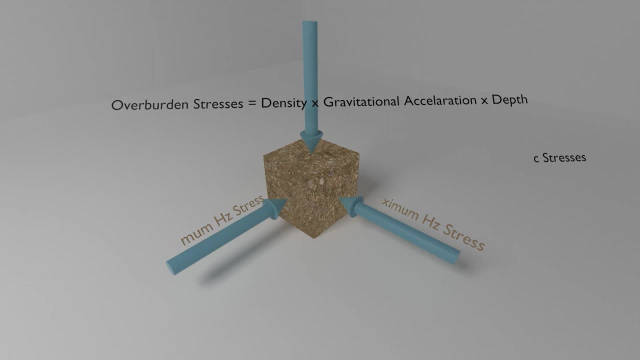 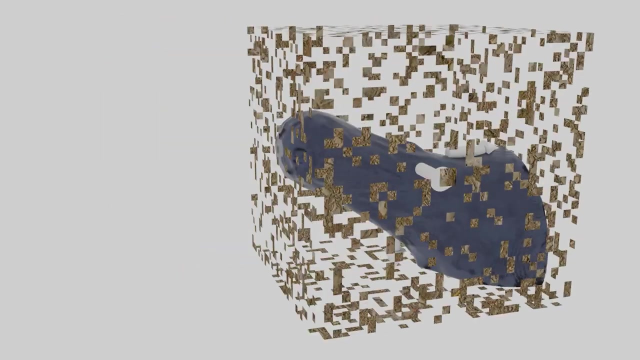 of the rock and fluids above from the surface till our tube. the horizontal stresses calculation is a bit complicated and is affected by three main stresses: the overburden stress itself. the poor pressure resulting from the fluid inside the poor spaces of the rock trying to escape. and 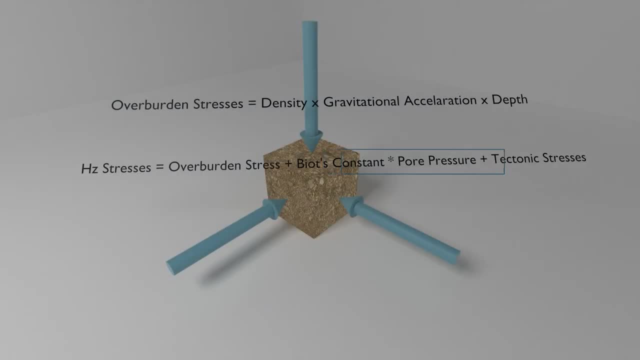 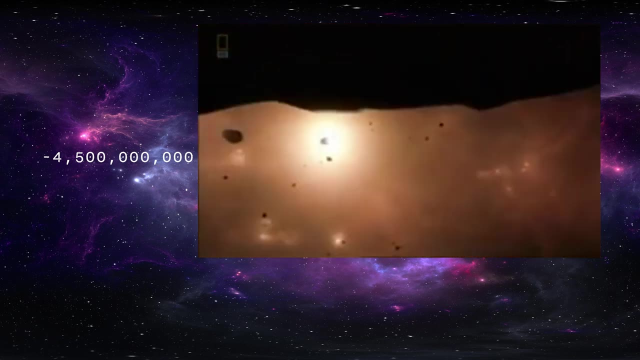 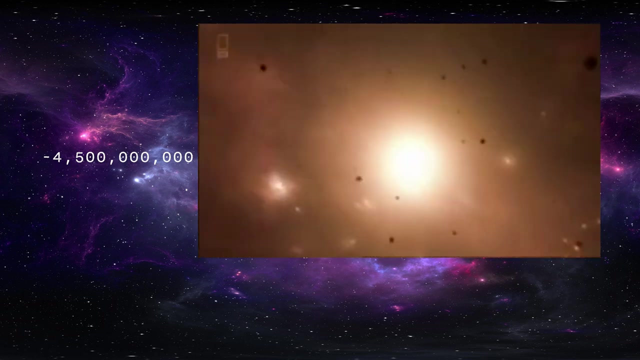 pushing the rock outwards. and finally, the tectonic stresses. in order to explain the tectonic stresses, we need to go back 4.5 billion years ago, when the earth was formed. it may be hard to believe that something as complex as a planet is formed with nothing but dust and rocks surrounding our newborn. 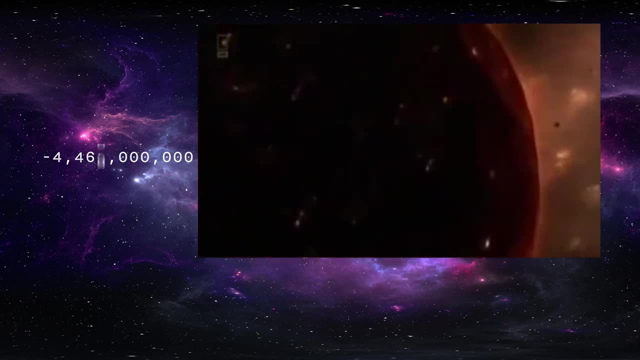 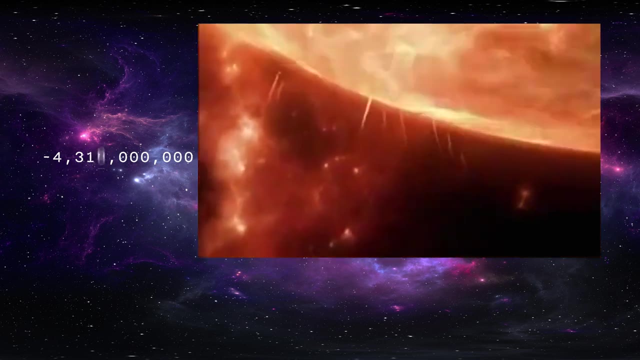 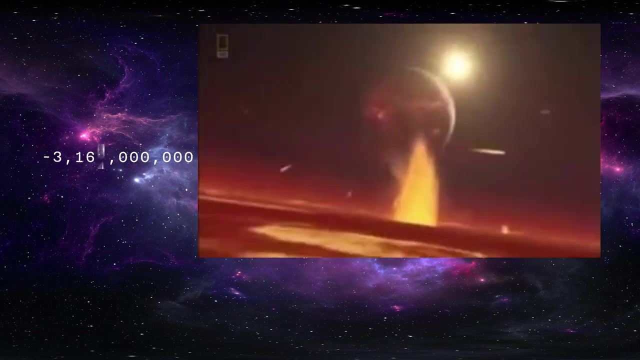 star the sun over millions of years. gravity pulls this rocks together to form the earth. back then, our newly born planet was simply a boiling ball of liquid rock with no solid surface, just endless ocean of life. a young planet called rhea, in the size of mars, then heads straight to earth and collide with it. 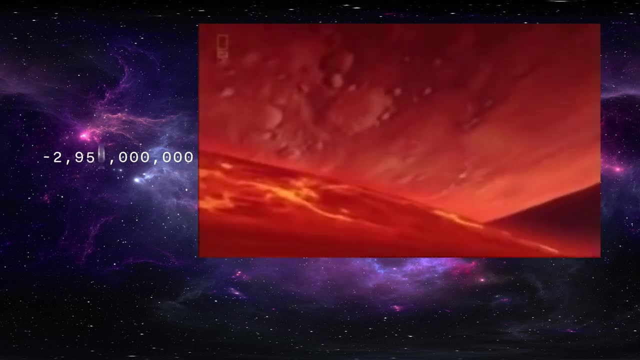 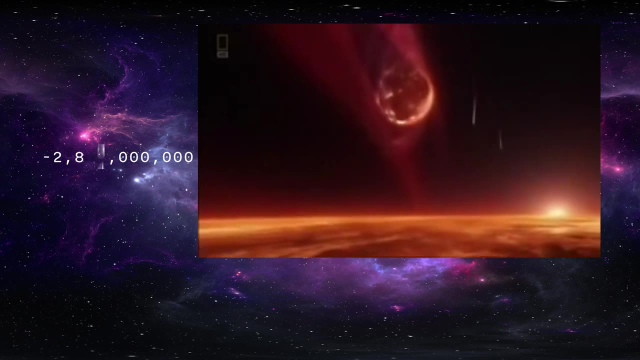 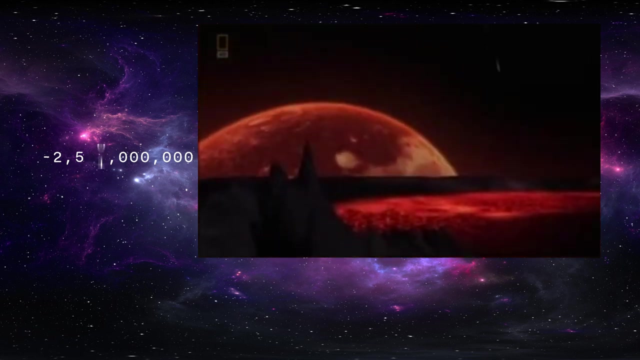 pushing it to its current course away from the sun and causes the formation of our moon. the moon is formed from the debris blasting out to space from the collision and circling earth, and while the moon is being formed, earth's surface started cooling down and forming its crust, and with any surface that has been cooled and solidified. 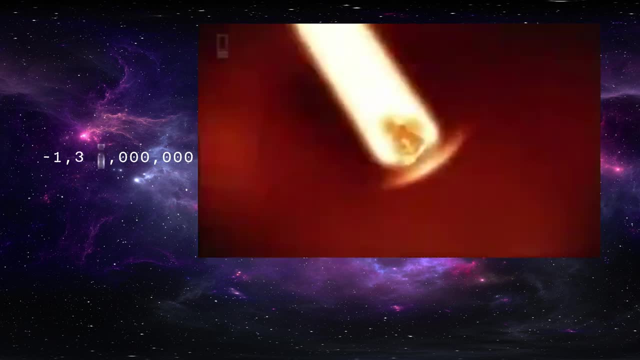 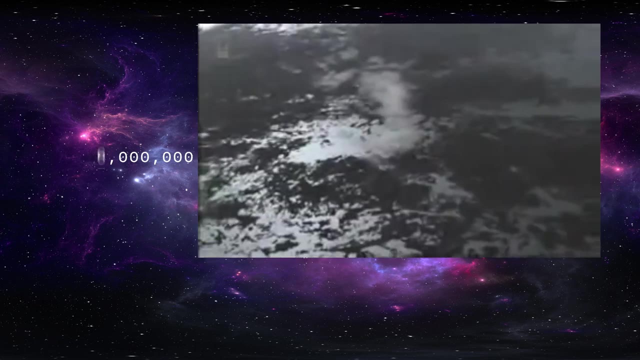 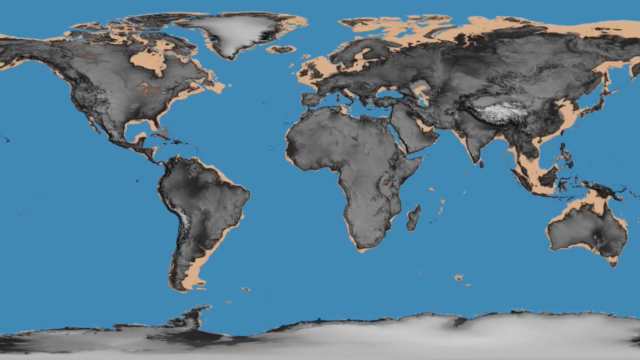 through time, cracks have been generated with water introduced to our planet. somehow, the shape of surface map we know now started to take place. now, looking at the world's map that we currently know, and if you take away the blue oceans and drain them away from the map, what we will see is not 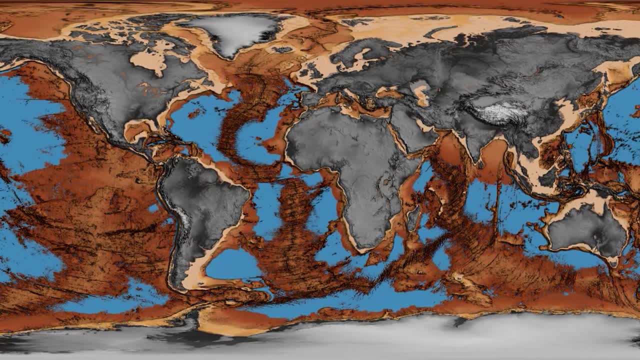 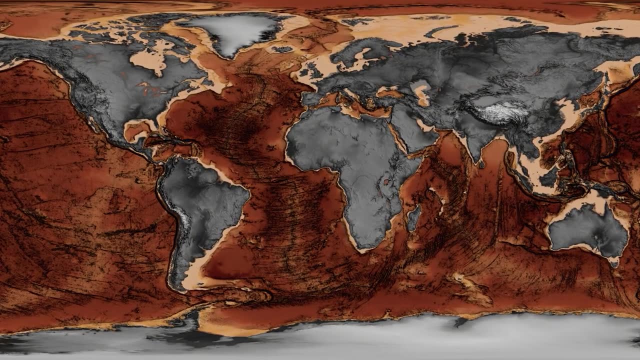 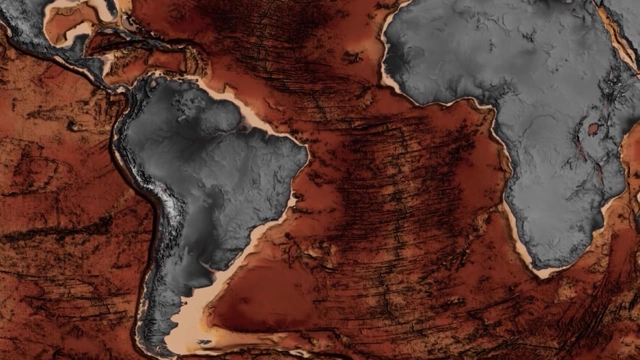 a flat sandy surface, as we may think, but rather a very active area with giant mountains and the volcanoes, creeks, peaks and valleys and earthquakes. if we zoom in, for example, in the middle of the pacific, we can see a massive crack in the crust. this is not the only crack in the crust. as a 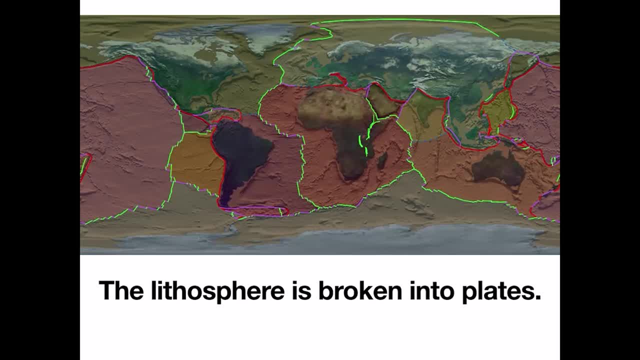 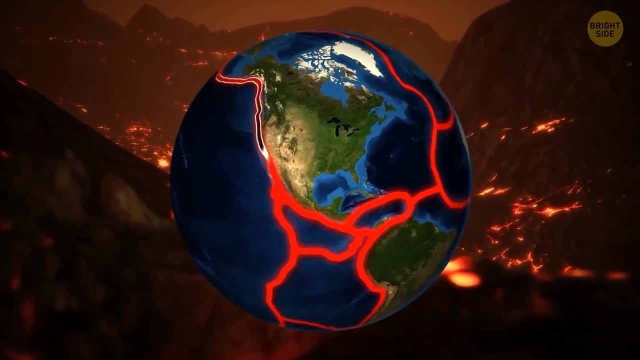 matter of fact, the crust is all broken down into pieces, and these pieces we call plates. now, those plates are floating over a gooey, semi-liquid layer of the upper mantle called the asthenosphere and, in case you don't know, our earth is considered a very high level of water. 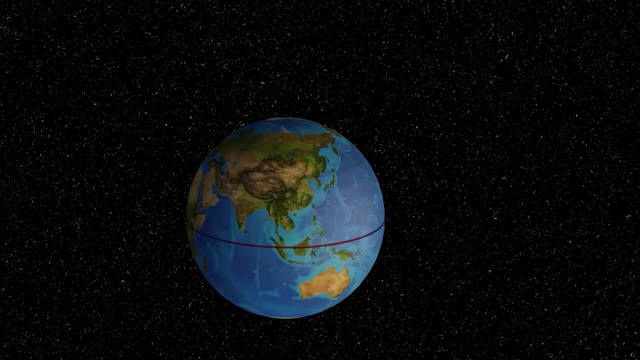 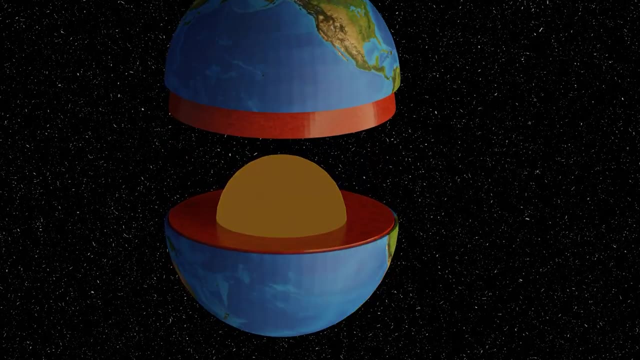 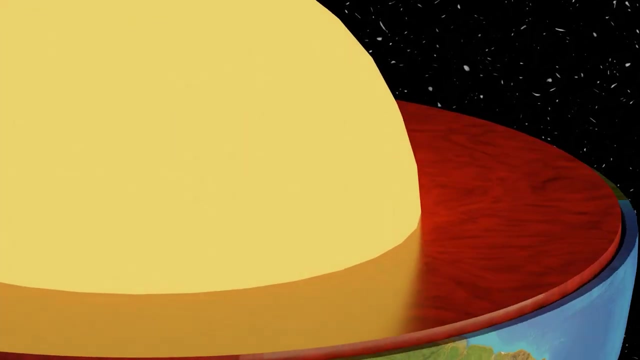 the crust is made up of different layers: the core, the mantle and the crust. scientists believe the core is mainly iron and nickel, as they are heavier minerals, so they sink down to the core, while the lighter minerals, such as silica, floats on surface, hence why the crust is mainly silica. 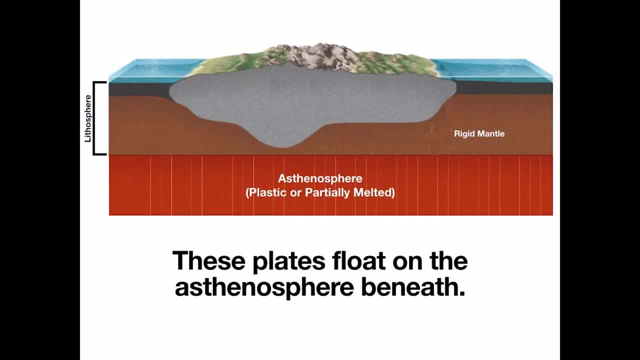 the crust as well as any solid surface of the upper mantle are called the lithosphere, and the lithosphere is pretty much all the rigid part of the mantle as well as the crust, while the asthenosphere is whatever semi-plastic or plastic or partially melted layer underneath. and when it comes to the crust, there are two types of crust. 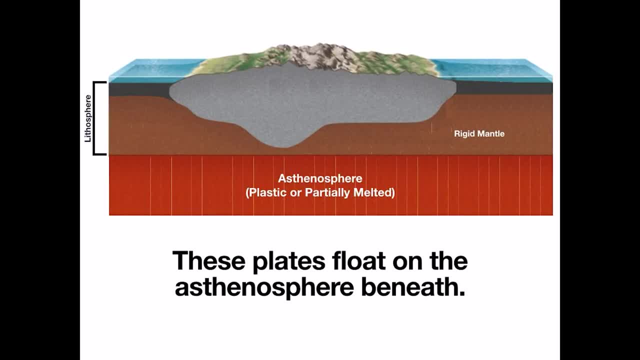 the continental crust and the oceanic crust. the continental crust usually thicker and lighter because it's formed from a sediment rocks precipitating on top of the oceanic crust. the oceanic crust on the other side is usually denser and thinner and lies underneath the ocean. 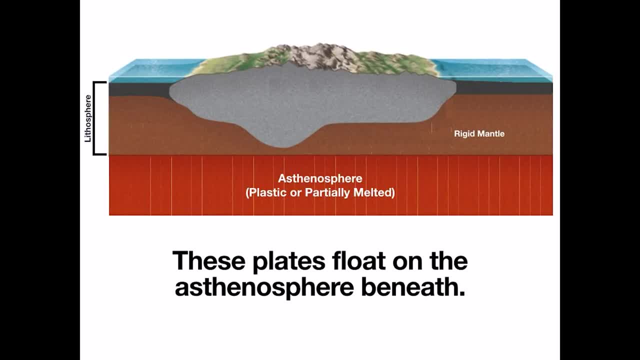 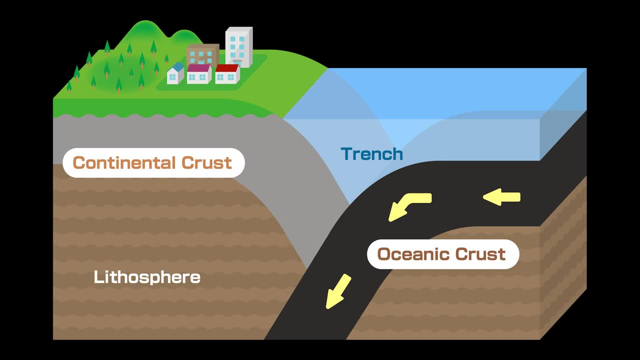 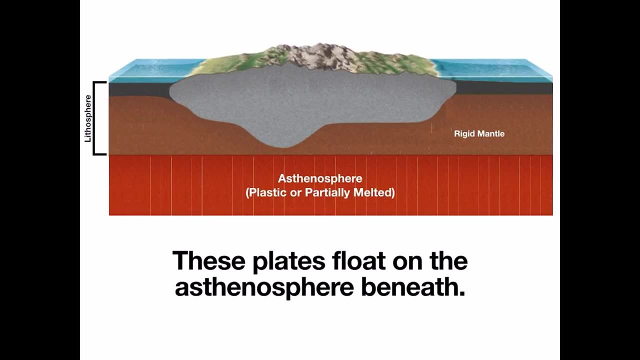 and it's mainly made out of basalt rock, hence why it's denser. and when those two meet, the denser crust sink below the lighter crust and burn out into the asthenosphere. now this gooey, semi-liquid part called the asthenosphere is continuously moving due to the convection process, where cold. 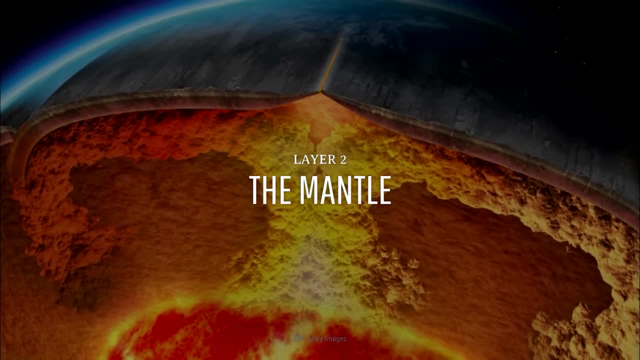 material. as it gets colder, it's denser and thinner. and when it gets colder it's denser and thinner. and when it gets colder it's denser and thinner and thinner. and when it gets colder it's denser and thinner increases. so it sinks to the bottom, while hot magma rises to the surface as it gets less dense. 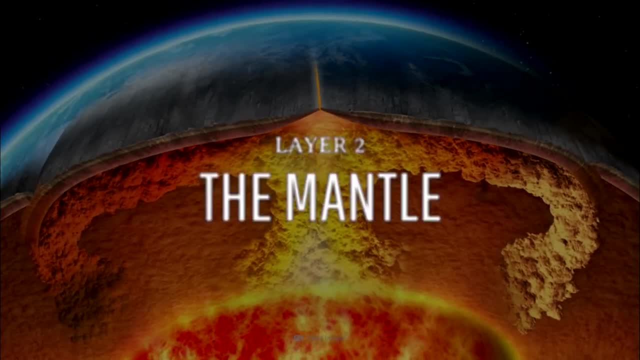 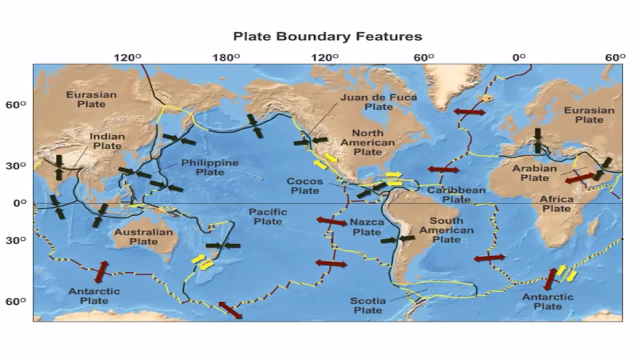 this movement is pretty much the drive for the plate movement above. so if we go back to the world plates map, we will find lots of action at the places where the plates meet and that's where we find all of our earthquakes and where we can find all of 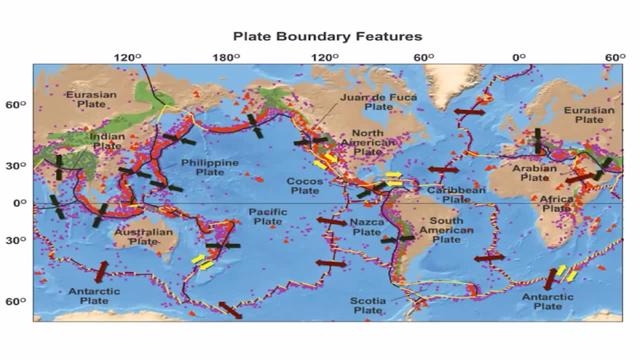 earth's volcanoes, and also where we find most of earth's active mountain ranges- and the interaction between the plates at the plate boundaries are guided by the direction of the movement of the plates. these directions, here indicated by the arrows in this map and based on the directions 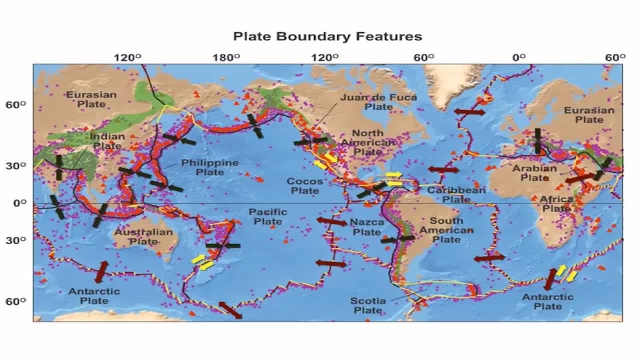 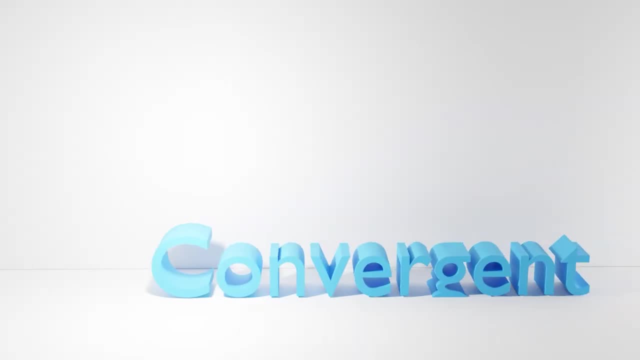 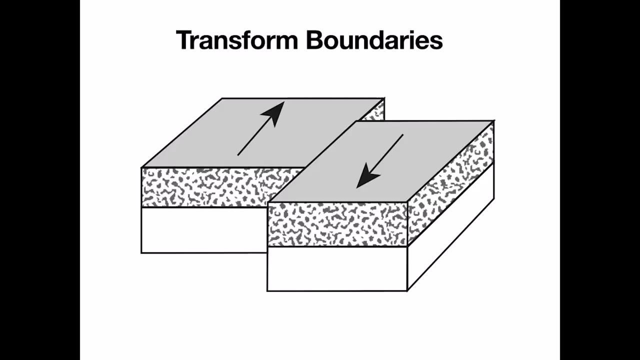 we can summarize all the interaction between the plate at the plate boundaries into three different types: transform, and that occurs as the plates slide past one another. conversion boundaries and the plates are colliding with each other. in transform boundaries, as the plates slide past one another, a high pressure and friction happens. 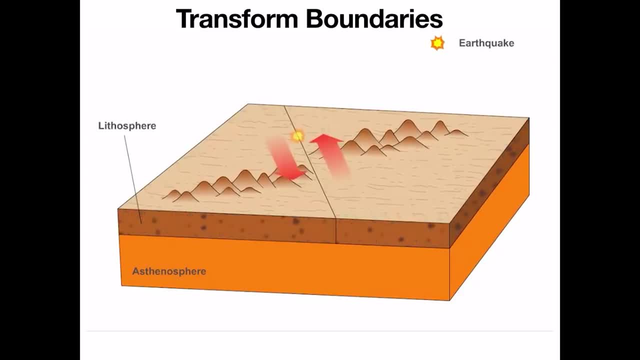 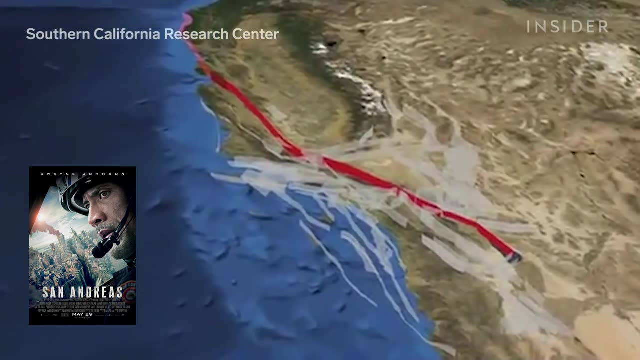 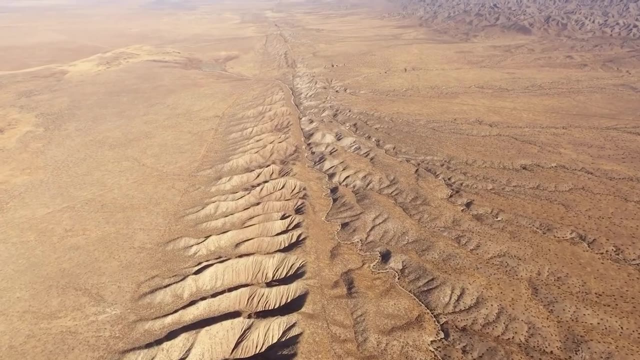 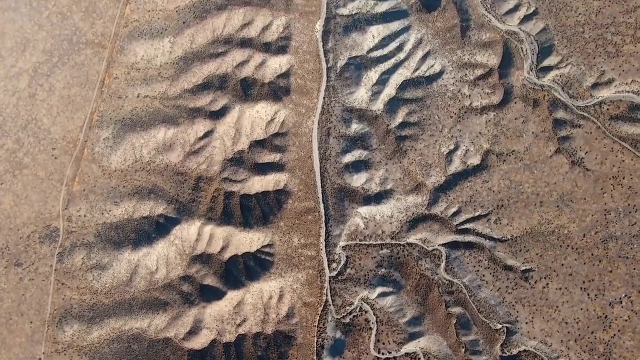 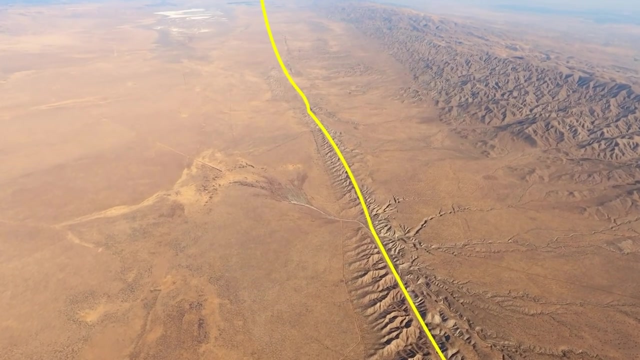 between the rock, which causes earthquakes, but they don't tend to have volcanoes or major mountain ranges. a famous example of transform boundaries is the san andreas fall. so one of the cases where it happens in this case is to have a vespa situation, where the plates are moving from one side to the other. 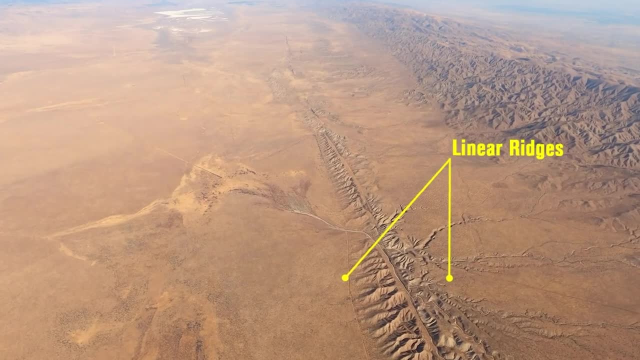 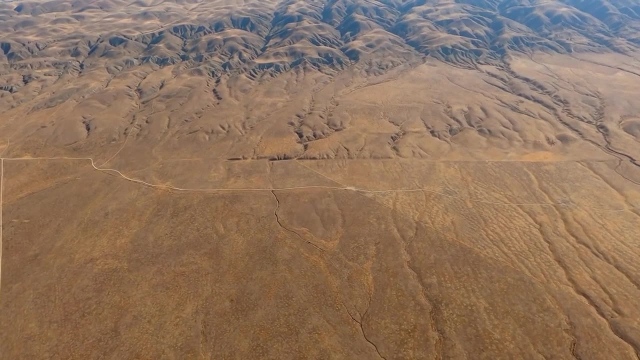 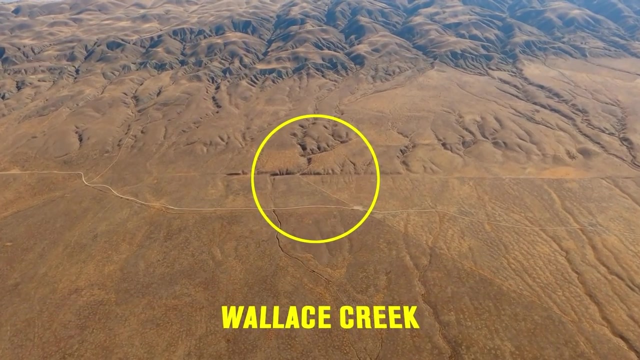 so we can pulled in the plateau to try and affect the portion under which the plate is farther than the changes theинг of the plates and their density. also we have in this case the point of the plate axis. like the crossing of the plateau is very specific, for example if a plate is moving from one side to the other. then we can, left over the plate to over, come forward over the plate area where it was before and over it necessary to do so. this example occurs all the time that the plate axis happens to be on the bottom and right side. to the other side, that it is in our position and over the middle and left side. it's privilege, basically an informality, that we can just let go away from each other and move forward along theよね. parents are helping so that they